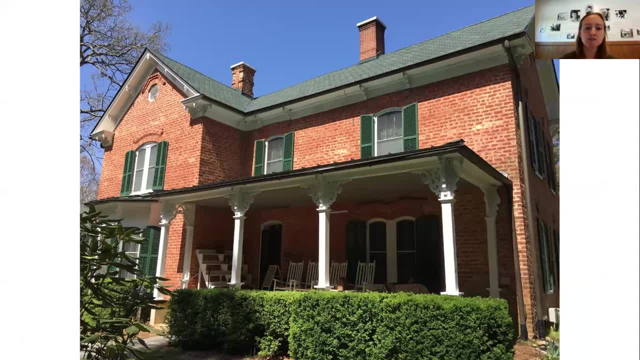 So it was Sally and her two sons living here in the house and they were running the farm. they had livestock, they had crops. they were always busy doing farm work, but farming doesn't always make enough money to live off of, so they needed a way to bring in more money, and Sally really couldn't. 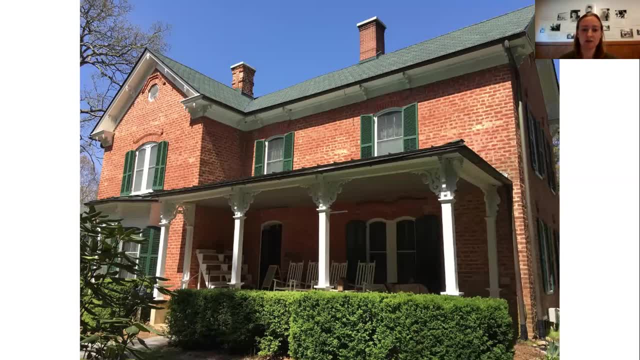 go just get a job, with her sons living at home. so she decided to open up this house for summer guests to live in. It was kind of boarding house. that was pretty common back then, especially in the area we live in in Henderson County. It's in the mountains. people would come up from Florida and Georgia. 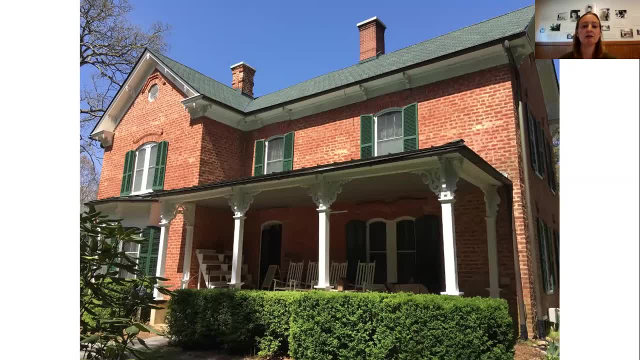 and South Carolina to get away from the heat and the humidity and the mosquitoes, and they would find a place to stay during the summer. Now, if you were really rich, you could afford a summer house, and the area of Flat Rock here in our county was known for people who were really rich and 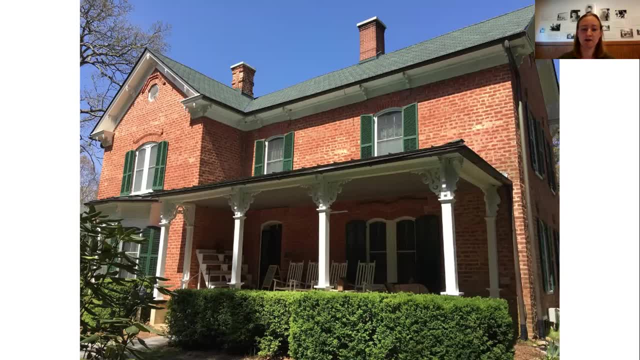 especially from Charleston, coming up and buying summer houses here. but if you didn't have quite enough money to buy another house, you would find a boarding house to stay in, such as this one. So people would come up, mostly people from Florida came to stay at the Johnson farm and at first they 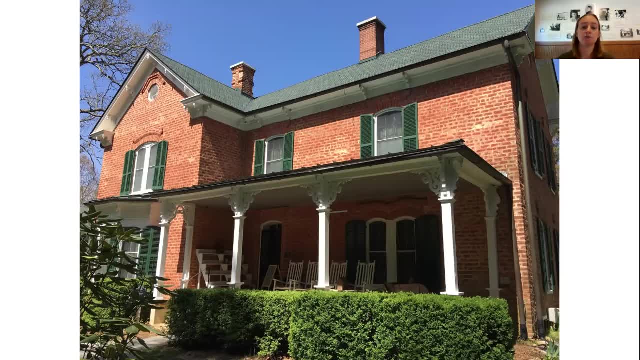 paid five dollars a week to stay here and that included three meals a day cooked by Sally Johnson herself. and people that stayed here had so much fun, especially the children. For the adults it was really kind of a relaxing vacation, but for the kids they would run around outside all day. 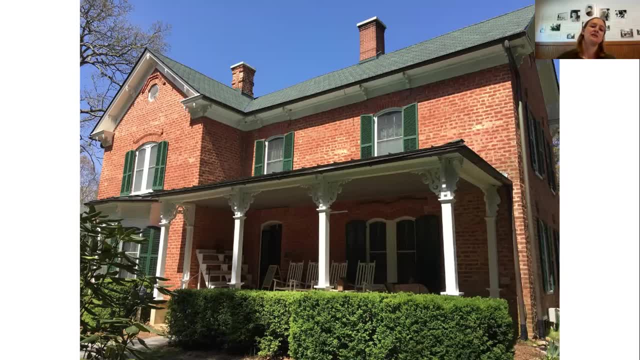 Vernon and Leander would take them around and teach them how to take care of the animals and help them help. they would teach the kids how to help them with their farm work like milking a cow and things like that. So kids especially had a lot of fun here. So that's a little bit of background. 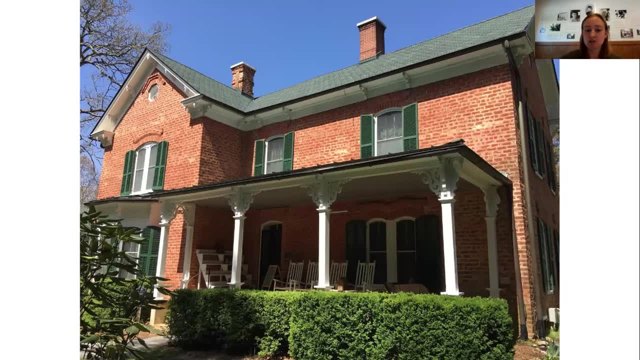 information to give you, but I want to start showing you some of those historical events that I've been told about. So one of the things that we'll do today is we'll show you some historical photographs, and I want you all to think like historians, which means, uh, to think like people that study history. 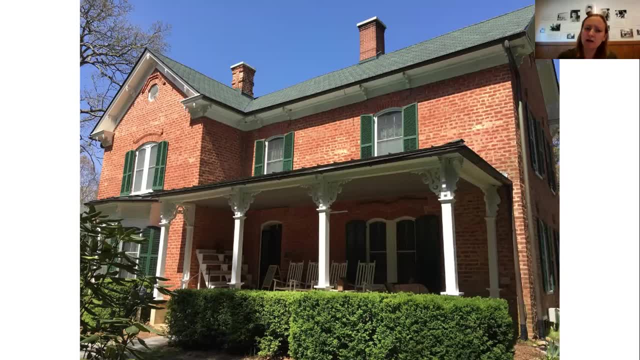 They're given a photograph. they might not know anything about the photograph, but just by looking at it, looking at the clothes people are wearing, if they can identify any of the people in it, they can kind of start to make some educated guesses about what is going on in the photograph. so some of these 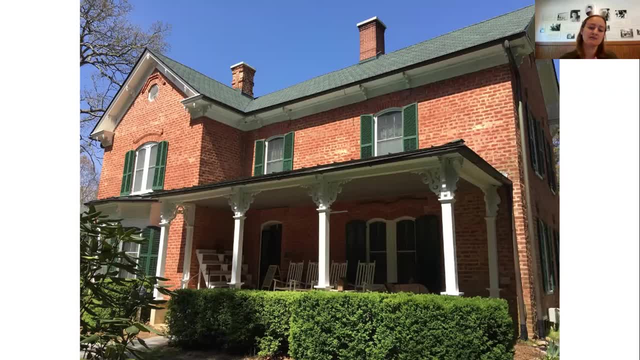 you might not know anything about the photograph of ask some major questions as you look at each picture. Where was the picture taken? If you can tell if you've been here to the farm before, it'll help, but you don't have to have been here to. 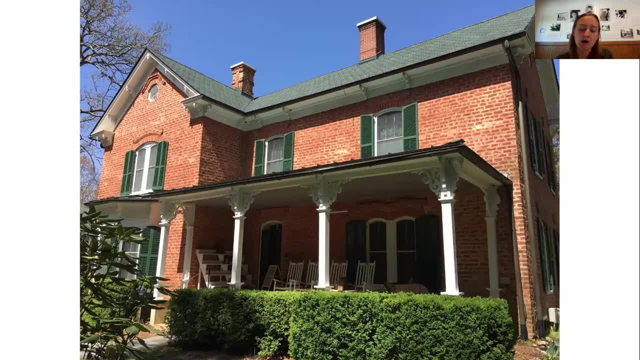 to be able to do this. Who do we think the people are? And maybe not necessarily their names, but do we think they lived here? Do we think they worked here? Do they think they, do we think they were summer guests that stayed here? Why do we think the picture was taken? Why? 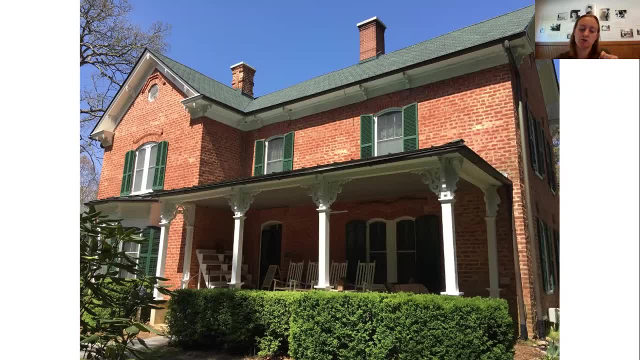 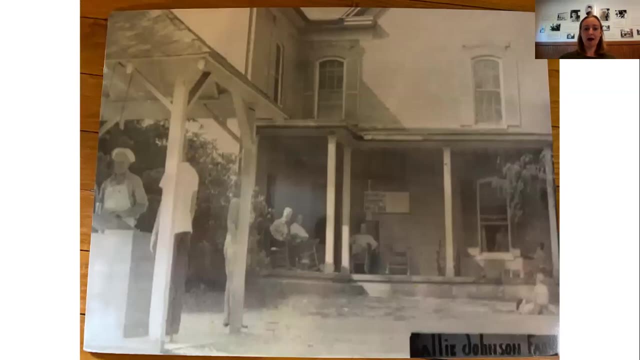 would a why would a photographer say, oh, I'm going to take a picture right now of this moment in time. And finally, what are they doing? What are they doing in the photograph? So, to start with, we have this picture here and this is the back of the house I just showed you. 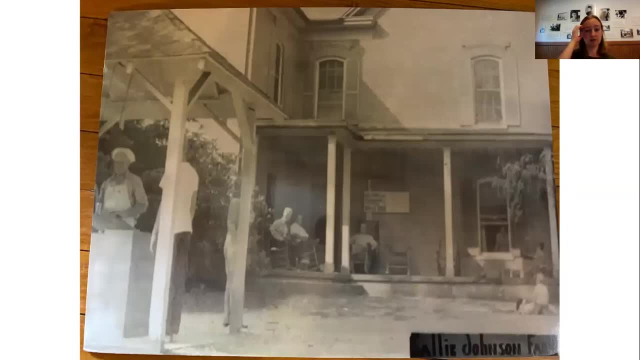 When people arrived at the farm, they would actually come via the back door, because the driveway came up and dropped people off right here. So we have the back porch, We have a well over here. that's still here at the farm today. So what do you notice? 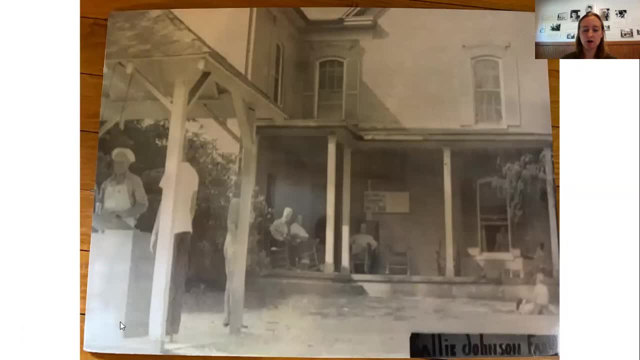 about this picture? Who do we think these people are? What are they doing? Why did the person take the photograph? And I can only identify one person in this photograph for sure. I know that this is Leander Johnson over here, because I know what he looked like And he is at the. well, And, if you can, 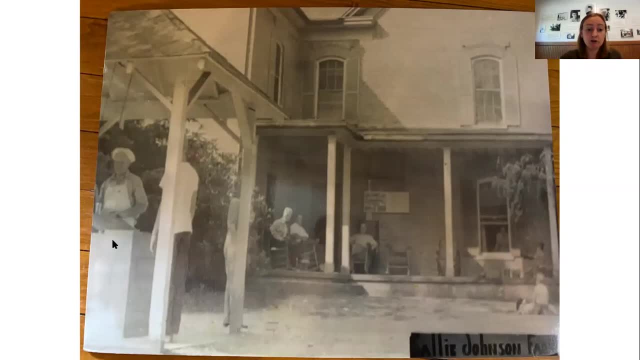 tell he's taking the cover off the well and he's going to get some water out of the well. He's wearing an apron, So I bet he's going back in the kitchen with that water or maybe taking the water to the animals. But he's wearing an apron which shows he is doing some kind of work, And I know. 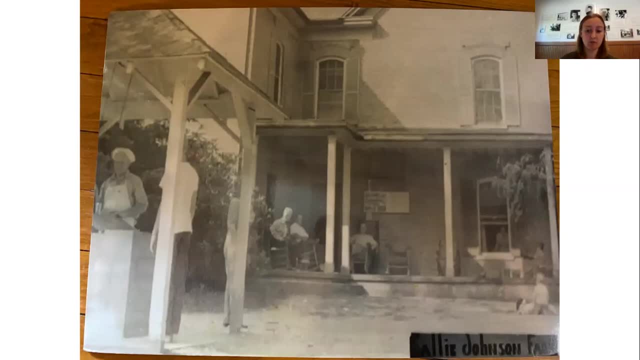 that he helped in the kitchen a lot, So that's why I think he was probably going to the kitchen Now on. And the porch? Who do we think these people are? I think they are summer guests that were staying here. because they're sitting there, They're rocking in their rocking chairs, They're relaxing. 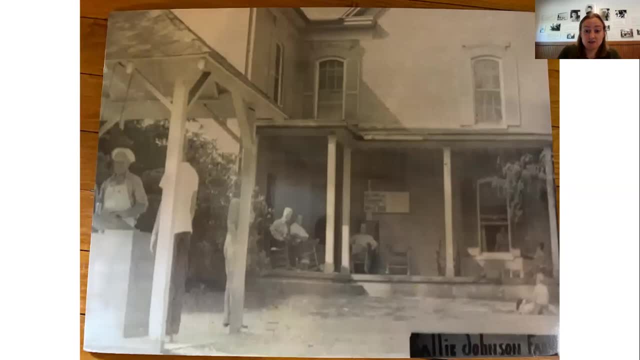 And that is exactly what a lot of the guests did. They would sit on this porch and they would just enjoy being outside. We see a woman here- I'm not entirely sure who she is. We see a child here playing with a dog, And we see some younger people here as well watching. 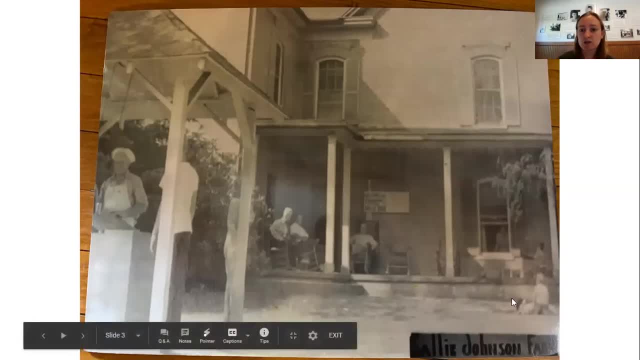 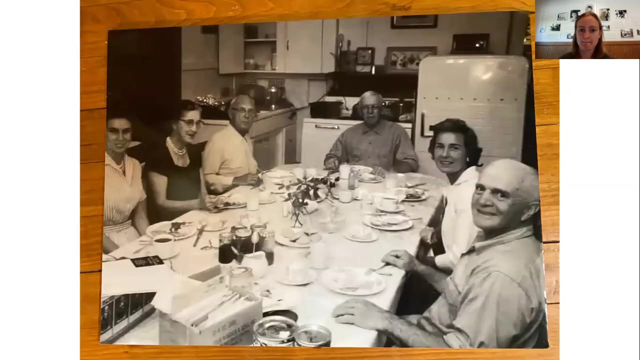 Leander. I think the photographer took this picture just to kind of capture a moment in time and show what life was like during a summer day here at the Johnson Boarding House. Now this picture Again. ask yourself, who do we think these people are? 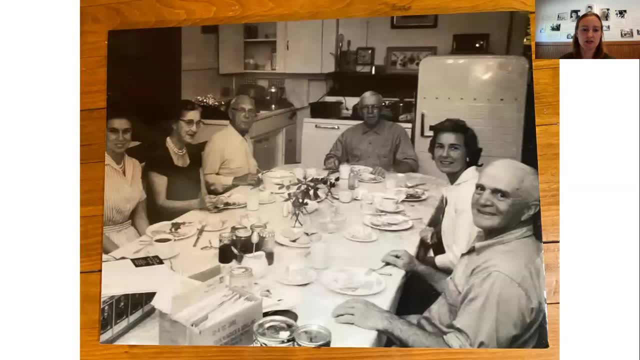 What are they doing? Why did the photographer take it Now? I know that this picture was taken a little bit after the boarding house days, And I know that because this is in the dining room now. But the dining room while the summer guests were here did not have a kitchen in it. The 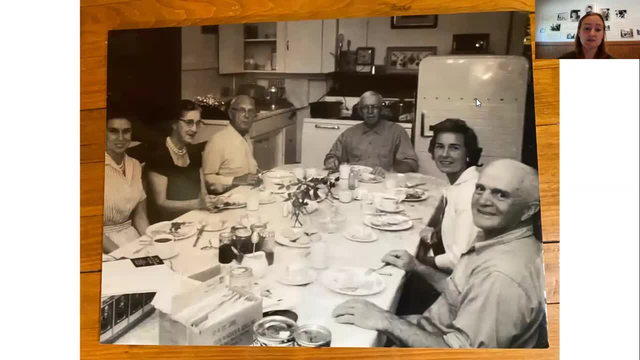 kitchen was in a separate room, But once Sally died and once the brothers kind of stopped the boarding house business, they moved some of the kitchen appliances in here, so it would all be in one room. I know that this is Leander here. I know that this is Vernon. I'm not sure if this is. 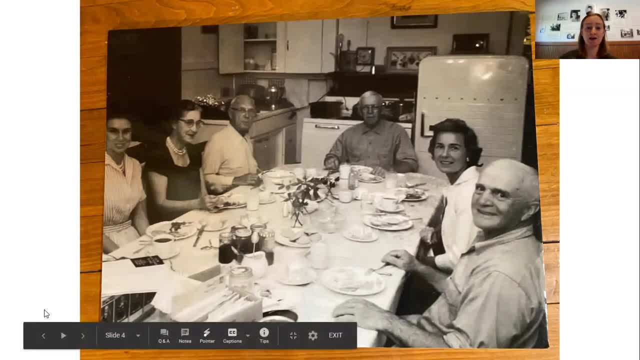 Leander. I'm not sure who the other people are, Because back then, when they had photographs printed, they did not write down who was in the picture. So this is my plea to you all: If you ever print photographs- which I don't know if anyone ever even does that anymore- But if you. 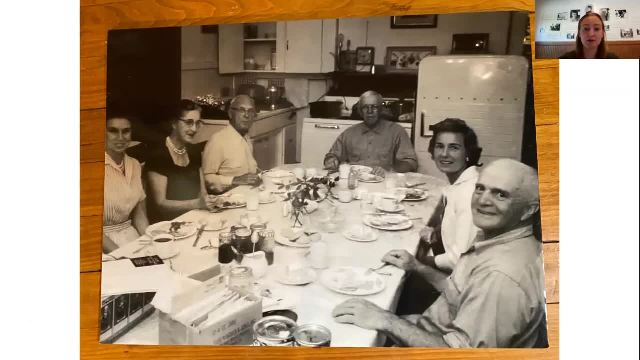 print photographs. please, please, please, write on the back of it in pencil who is in the photograph, so that years from now, people looking at the photograph can know who is in the picture, Because I would love to know who is in all of these pictures. 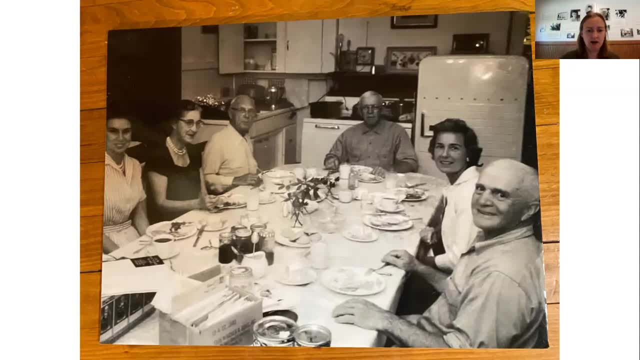 What are they doing here? They're obviously eating. I have many students that have looked at this picture that think it's breakfast, because we have biscuits, We have lots of jellies, We have coffee And I think they're drinking milk over here. And one interesting part of this picture: 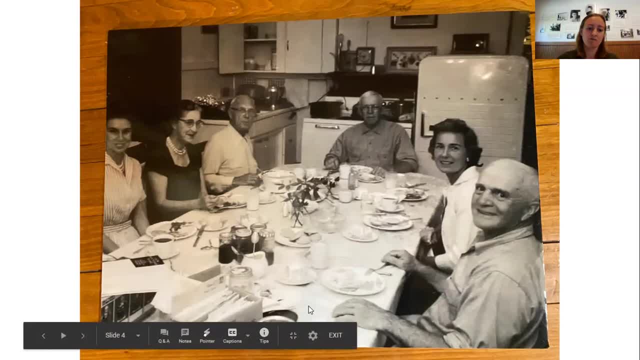 look at this box down here with all these cards. Vernon and Leander got so many different cards. They love to send letters to people, Leander especially, and they got mail in return, And we still have a lot of letters. So I'm going to show you a little bit of a picture of this. 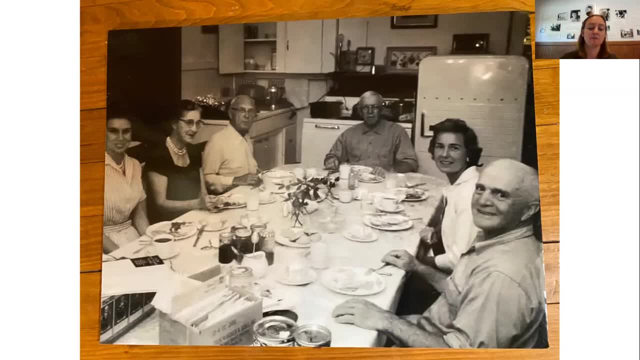 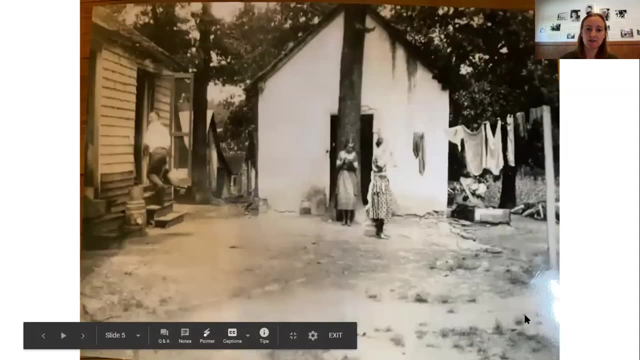 I think they will have a lot of these cards and envelopes and stamps that people sent to them. Now the next picture I have. this is the smokehouse here at the farm where they would hang and dry their meat. This is the kitchen before the current porch was added on. 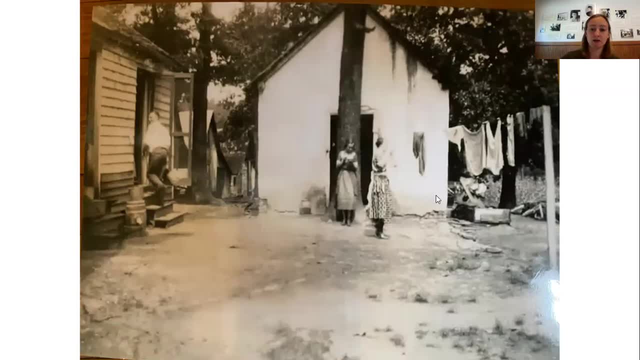 And if you've been here before, this might look a little bit different, because the smokehouse currently has an addition to it. The right-hand side has a building or kind of a few rooms added on for Etta Presley, who helped here as a housekeeper. 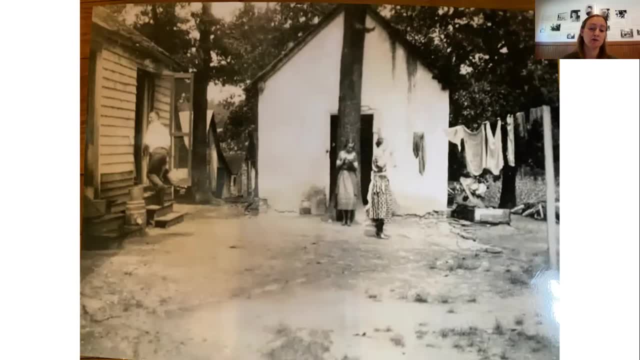 for many, many years. So this picture was taken before then. So I think this picture, my best guess would be that it was built or the picture was taken in the 1920s or early 1930s. Now I like 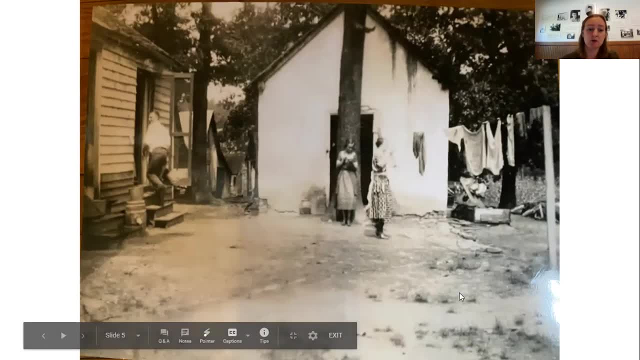 to ask with this question: who are these people? Do we think they were summer guests? My answer is no, I don't think they were summer guests. I don't think they were summer guests. I don't think they were guests mainly because they're wearing aprons. They're clearly doing work, These girls. 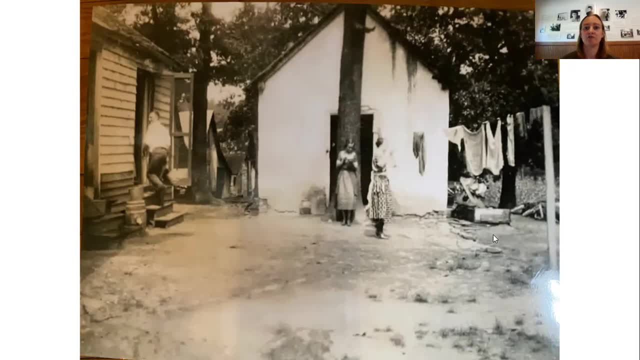 are hanging the laundry on the line to dry, and that would not have been something that the summer guests would have been expected to do. The hard work that was reserved for the Johnsons, and they would also hire people that lived here in the county to come and help with the cooking and the 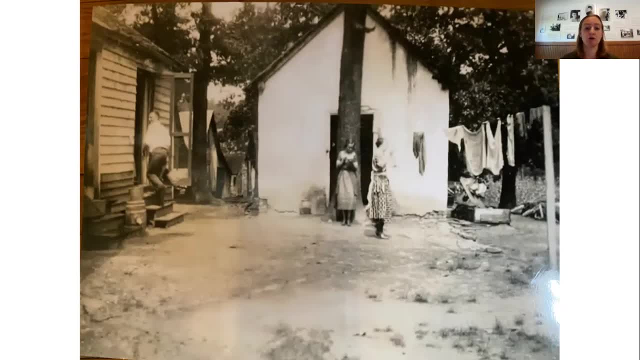 cleaning and the farm work, especially during the summer when it was busier here. So I think these are two young ladies- One of them is Etta- that helped here at the farm And it's kind of confusing A lot of people think. 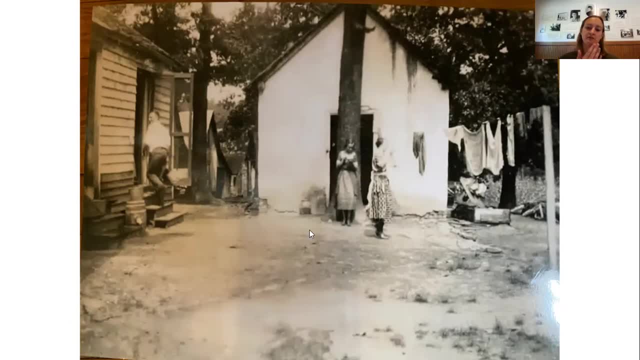 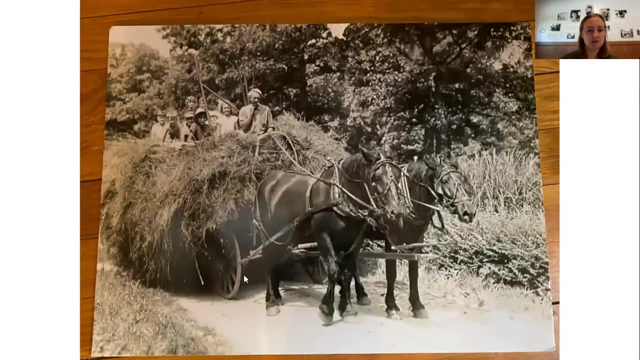 this tree is blocking the doorway. It's just the perspective of the photograph. You could actually walk behind the tree to get into the smokehouse. Here's another picture we have. So what's going on in this picture? We have Vernon Johnson there driving the horses on the wagon, and we have lots. 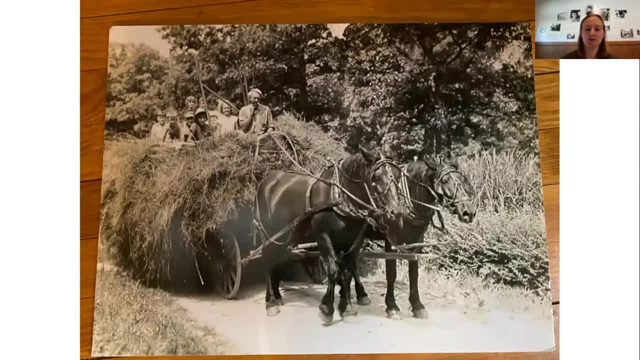 of kids that I think were staying home. So we have a little bit of a picture of him, And then we have a little bit of a picture of what he was doing here for the summer, And one day he said: just get on the wagon, We're going for a ride, which is something he did often, And there's a lot of hay. 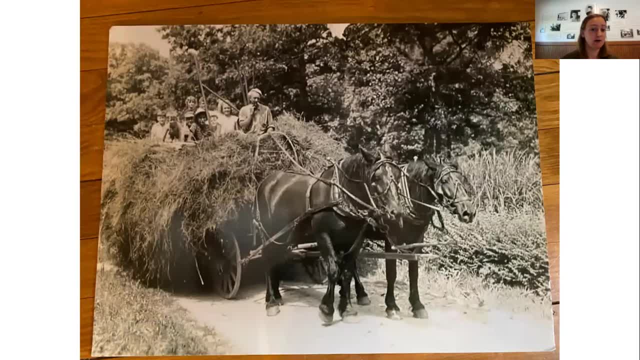 on that wagon. So I bet while they were having fun they were also probably stopping to feed the horses and the cows and the pigs and the animals that they had here at the farm as well. So he was putting the kids to work. But kids that stayed here, they remember riding on the wagon. They 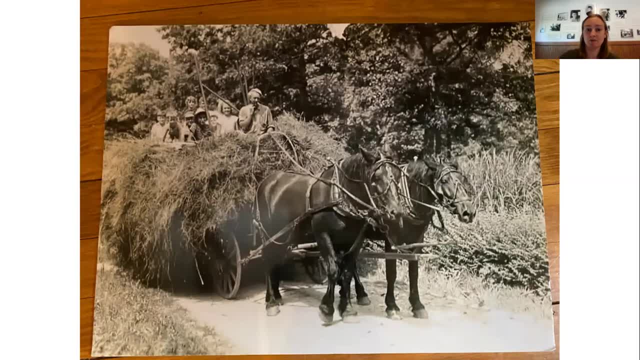 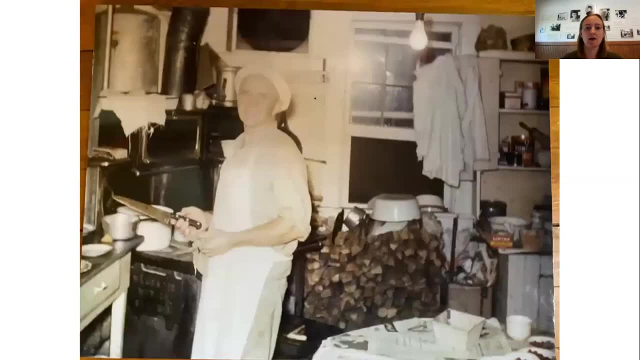 remember the Johnson brothers taking them around And showing them things on the farm and showing them how to feed the animals and take care of them. And then the last picture I have here: if you've been to the farm you might recognize the kitchen. 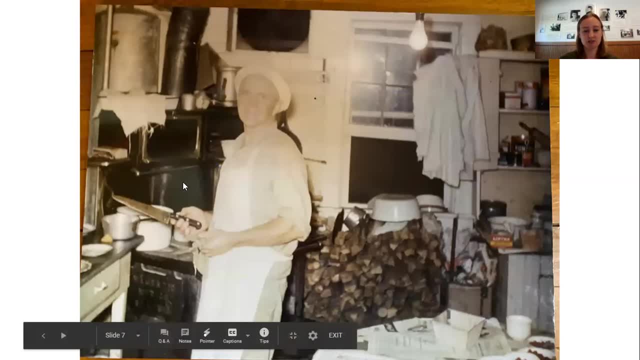 We still have the wood stove here that all of the cooking was done on. We no longer have the wood pile here, but that is how they would get that stove lit. And this is Leander Johnson, the other brother, And he again helped a lot in the kitchen. So we see him here again with the animals And we 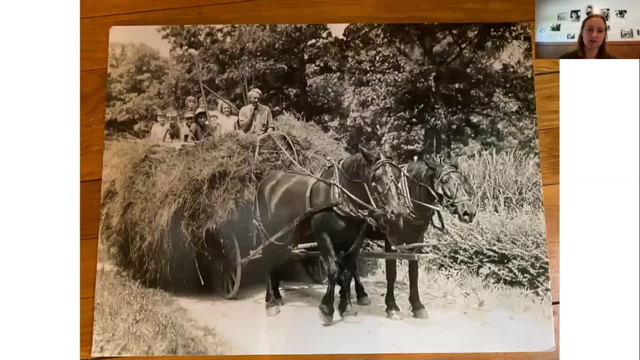 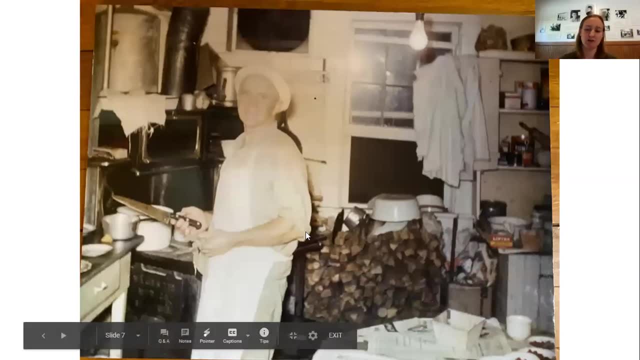 see him wearing the apron on, And both brothers. let's see in both of these pictures. you can see they always wore this little white sailor's hat. Pretty much in every picture we have of them that's what they're wearing. So Leander helped in the kitchen. A few things to note in this kitchen. 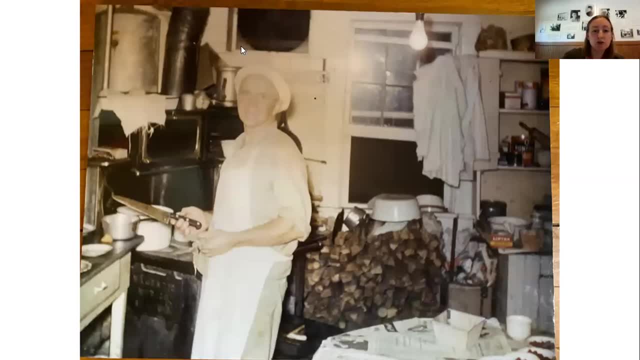 there was a fan up here, So currently we don't have the fan there, But for those of you that have been here and wondered what that hole in the wall was, there used to be a fan there. We have shutters over it now. 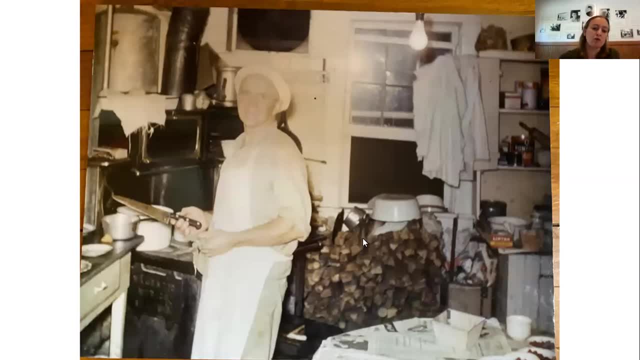 And then I like to ask people about this picture: What do you think are two things that you see that show that this picture was taken later in time than the other photographs, or at least some of the other photographs. And those two things are the light bulb, So it shows that there was. 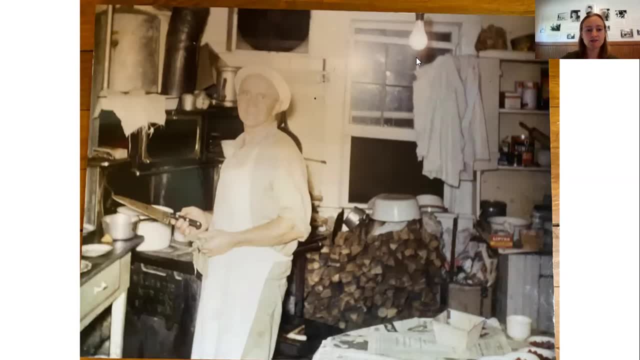 electricity, which they did not get until the 1920s- I think 1925 to be exact. So it was taken after that And this photograph is in color. The other photographs we saw were in black and white And that doesn't mean that people did not see color back then, but photographs could not.